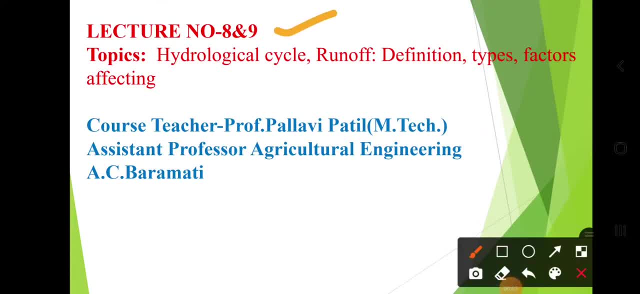 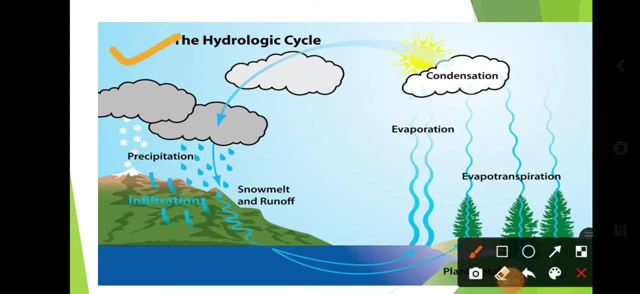 Hello student, today is our lecture number 8 and 9 and the topic is Hydrologic Cycle Runoff: Definition, Types and Factors Affecting the Paramotor. In that, firstly, we will see the Hydrologic Cycle. Hydrologic Cycle cycle means what? 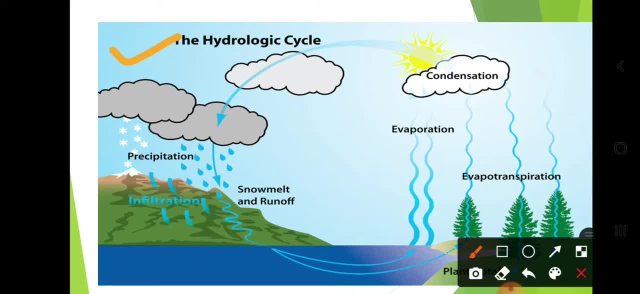 It is the sequence of event and that is repetitive itself. it is called as a cycle And in Hydrologic Cycle, what happens? Whatever the water present in river, seas and ocean, it will get evaporated and due to the evaporation of that water, from the water surface as well as 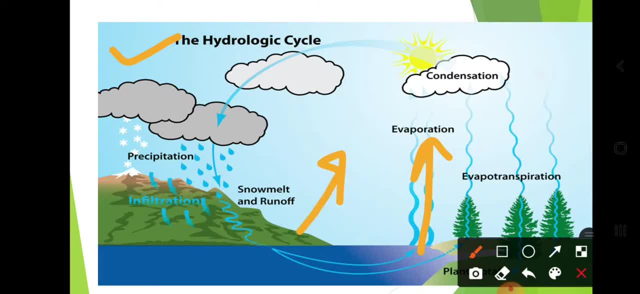 evaporation from the soil surface as well as the transpiration from the plant surface. it is called as evapotranspiration. There is a formation of the clouds and when the clouds received the cold air, there is a condensation and precipitation. precipitation means rainfall. 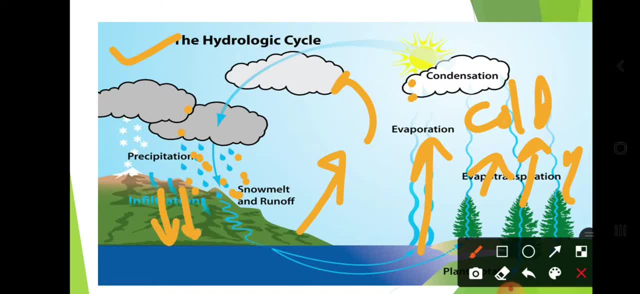 again that water. it will gets infiltrate into the ground. if there is a snow, there is a melting of the snow, then there is a runoff and again that water goes to rivers, sea and ocean. again there is a evaporation from the water surface, land surface, as well as evapotranspiration from the 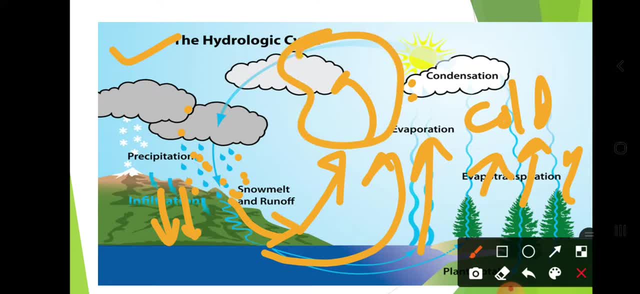 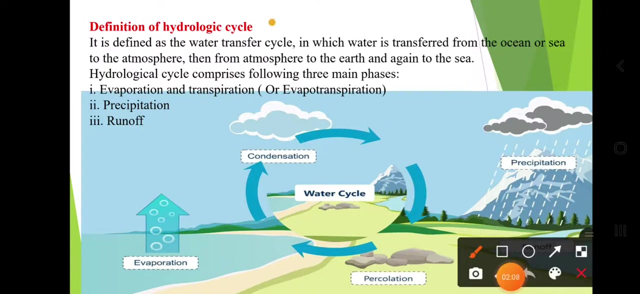 plant surface, there is a formation of the clouds. if the clouds receive the air- cold air- there is a condensation, then there is a precipitation. means this is sequence of event are repetitive and it is hydrologic cycle. then what is the definition of hydrologic cycle? it is very easy. 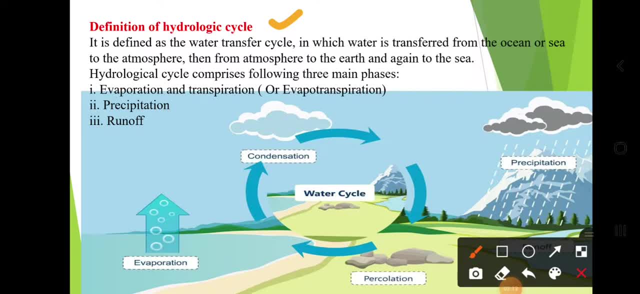 it is defined as the water transfer cycle. hydrologic cycle means water transfer cycle in which water is transferred from the ocean or sea to the atmosphere. hmm, means it is. hydrologic cycle is a water transfer cycle in which water is transferred from the ocean or sea to the atmosphere, then from the atmosphere to the earth and again to the sea. 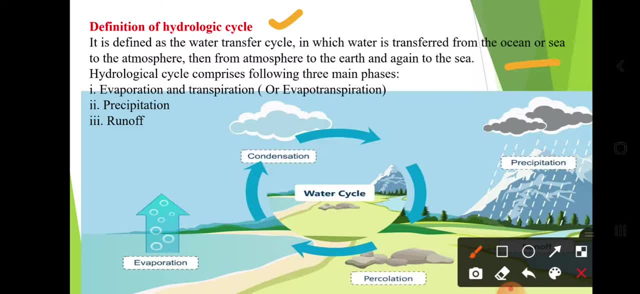 meaning the water transfer means what is water and water is無ond transfers- then flow through the atmosphere and again to place The ocean, the river. the ocean goes to the atmosphere again. When it goes to the atmosphere it comes back to the soil and goes back to the ocean. 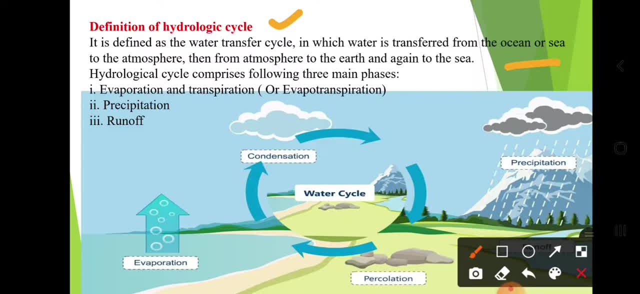 This is the hydrologic cycle And in that hydrologic cycle most important is evaporation and transpiration. It is also called as evapotranspiration. Precipitation means there are different types of precipitation: rain, sleet, hail, like that. 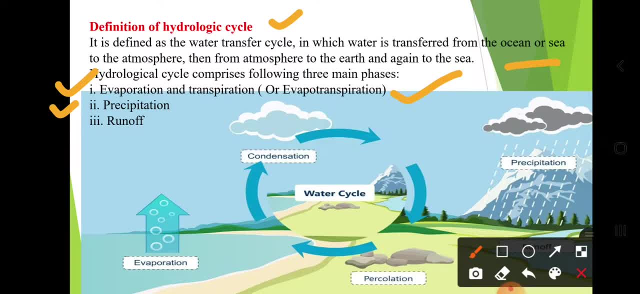 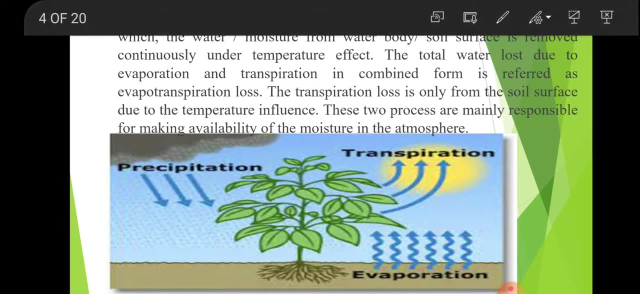 There are different, We will see in next slide. Then runoff. These three are most important: Evaporation, transpiration, evapotranspiration, precipitation and runoff. Now, evapotranspiration means what, Evaporation and transpiration means evapotranspiration. 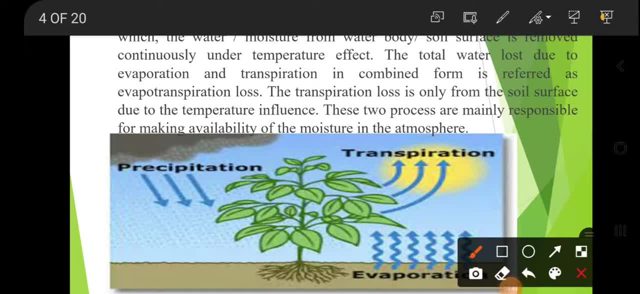 Okay When the water and moisture from water body, soil surface is removed continuously under temperature effect. When it is hot, when the temperature increases, it becomes a water vapor. Then water, water surface passes through the water, evaporation occurs. Evaporation occurs on the land. 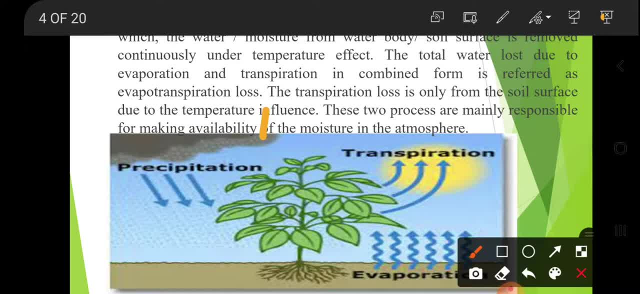 Evaporation occurs on the land. It is called as evapotranspiration. It means the water. it is evaporated due to the temperature effect. The total water lost due to evaporation and transpiration is combined or is referred as a evapotranspiration loss. 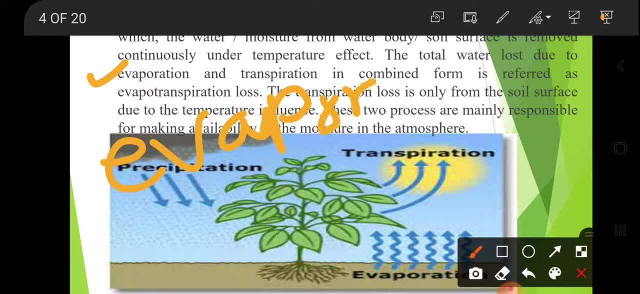 It means evaporation from the land surface plus transpiration from the plant tissues, plant leaf, plant roots. It is combinedly called as a evapotranspiration. The transpiration is a loss only from the soil surface due to temperature influence And the. these two processes are mainly responsible for making the availability of the moisture to the availability of the moisture in the atmosphere. 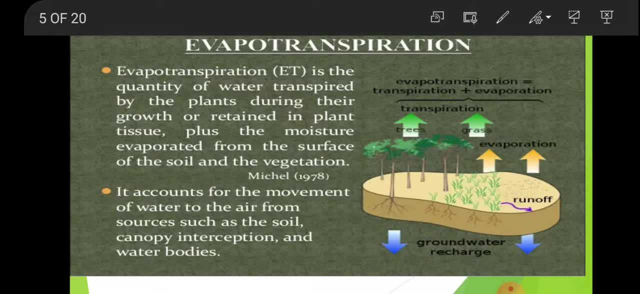 Now again this slide. it will explain clearly, Clearly, the evapotranspiration. Evapotranspiration is denoted by the letter ET. ET means what Evapotranspiration is the quantity of water transpired by the plants during their growth or retained in plant tissues, plus the moisture evaporated from the surface of the soil and vegetation. 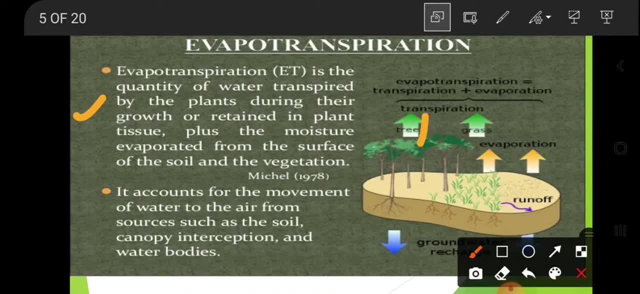 Mjhe Plantsya tishumadhun Plantsurface. Plantsurface Pani Evaporate otat Tasha waphe madhiru pantar hoto. Parat Surface varunpan evaporation hoto. 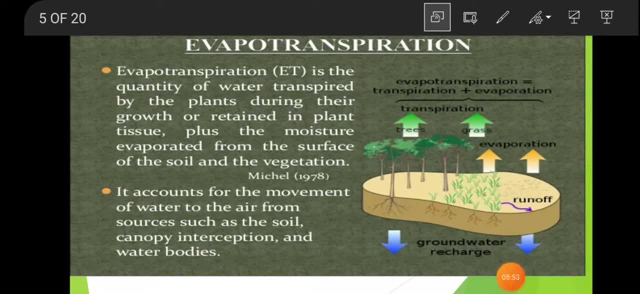 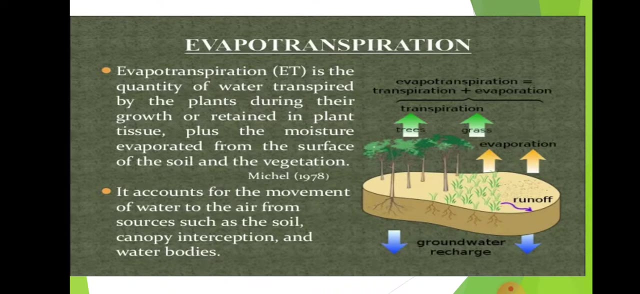 It is combinedly called as a evapotranspiration. It means transpiration plus evaporation. It is evapotranspiration. It accounts for the movement of water to the air from sources such as the soil, canopy, interception and water bodies. 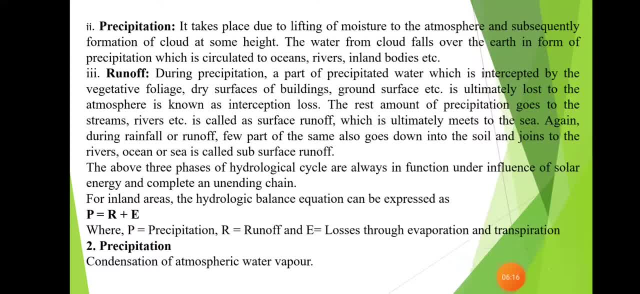 Now precipitation. The most important point is precipitation. It takes place due to lifting of moisture to the atmosphere and subsequently formation of clouds. at some height, The water from cloud falls over the earth in the form of precipitation, which is circulated to the ocean, rivers and island bodies. 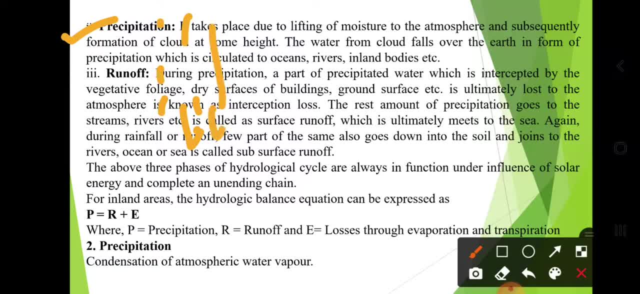 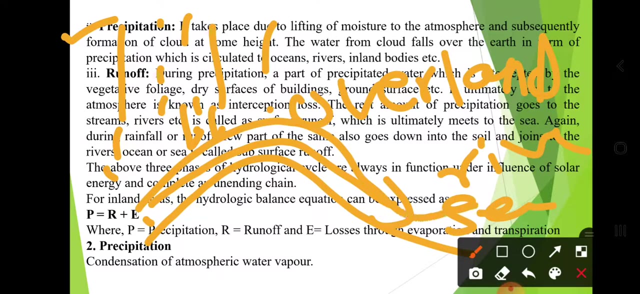 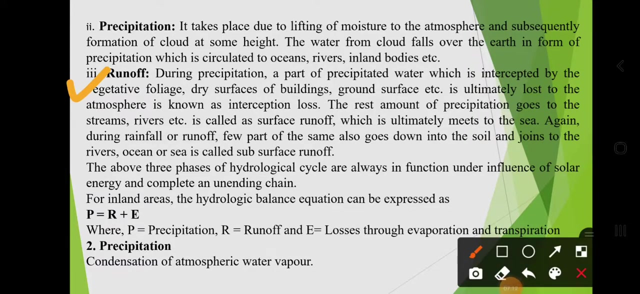 It will move away as a runoff overland flow, overland flow or runoff and it goes to the rivers, seas and ocean. Okay Means that water from atmosphere again goes to the rivers, oceans and sea, Then runoff during precipitation. a part of precipitated water is intercepted by vegetative foliage. dry surface of building round surface. 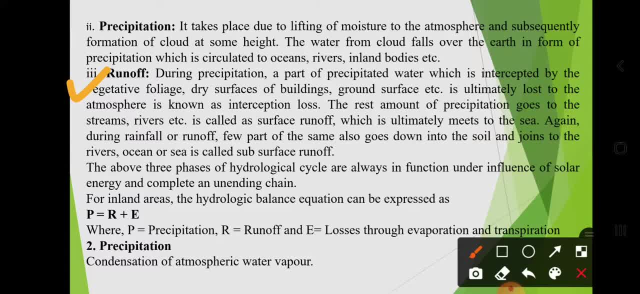 It is ultimately lost to the atmosphere is known as interception losses. Okay, Means that water from dry surface gets infiltrated, goes to the ground surface, goes to the buildings. It is an interception loss And means that during the monsoon, what happens to the water in the dry surface? 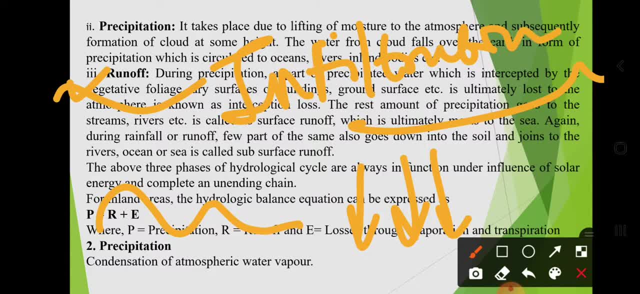 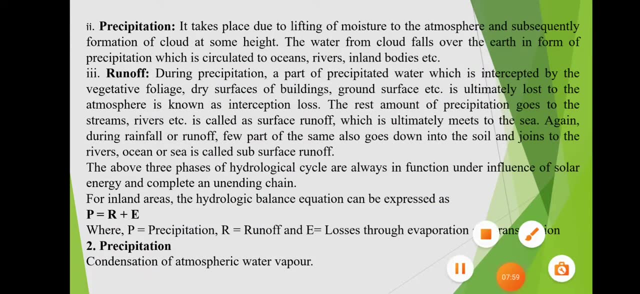 Infiltration of the water. It is the first entry of water into the soil. It is called as infiltration. After infiltration, whatever. there is a detention, storage are there. The soil become fully saturated. Saturation means what, Whatever the pore. 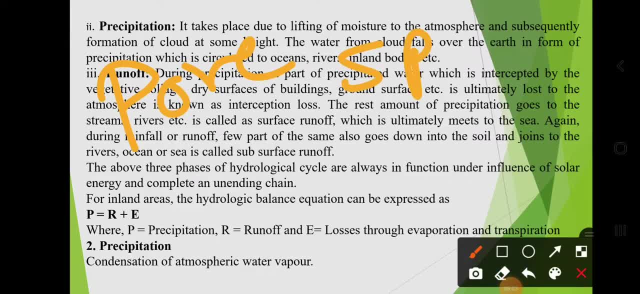 Pore spaces present in the soil. it is filled by water Wherever there was air in the soil. now what has happened? Water has settled And now the soil? it is not able to absorb the water Means, it is saturated. And from that saturated soil, the water still. the rain is falling. 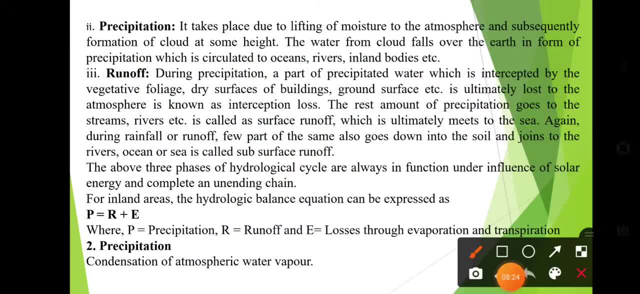 It is raining. The soil is completely saturated with water. Now that water cannot be absorbed, What does it mean? The soil is full, The soil is saturated, Now still the rain is falling with a higher intensity. There is a rainfall Pous padta chahi. 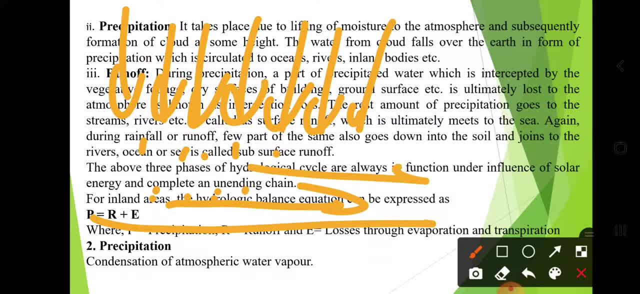 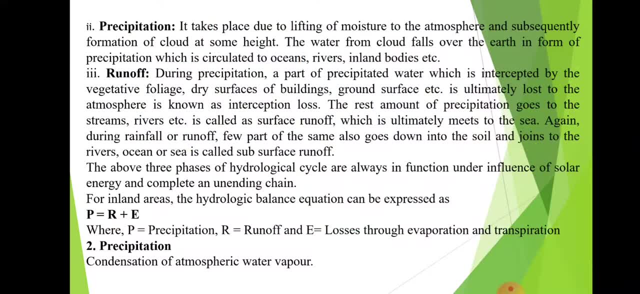 Soil purna saturate zhali hai. At that time, the water is moving over the surface and it is called as a surface runoff, And that water goes to the rivers, oceans and sea Means during the precipitation, a part of precipitated water which is intercepted by vegetative foliage. 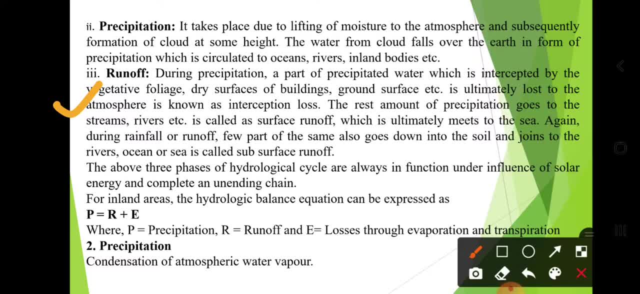 Dry surfaces of buildings, ground surface, etc. is ultimately lost to the atmosphere, Is known as interception loss. The rest amount of precipitation goes to the streams, rivers and ocean- Is called as a surface runoff, Which is ultimately meets to the sea again during rainfall or runoff. 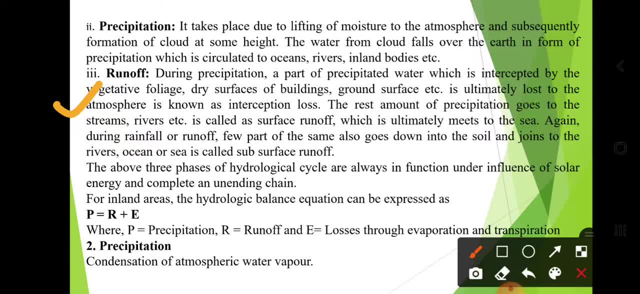 A few part of the same also goes down into the soil and joins to the rivers, ocean and sea. Soil purna saturate zhali hai. At that time, the water is still flowing with a higher intensity. There is a rain, There is aども. 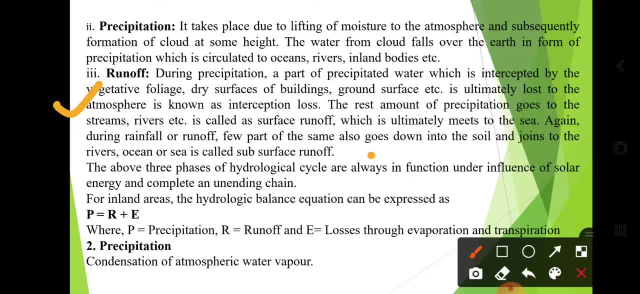 The soil is full, The water is also focusing the water on the surface. At that time three more phases of hydration, Or C is called as a subsurface runoff. The above three phases of hydrologic cycle are always in function under influence of solar energy and complete and uncompending. 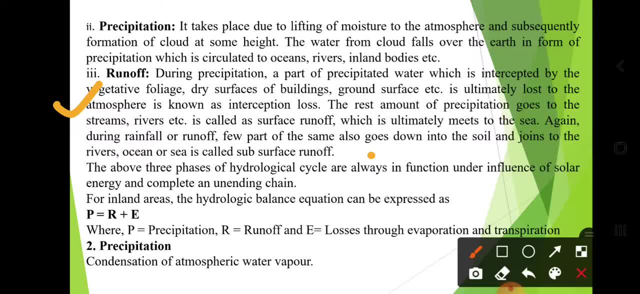 chain For oil and areas. the hydrologic balance equation can be expressed: P equal to r plus e. P means rainfall, Precipitation: Kitti pous, padta, Kitti pavispadna. whatever the rain it is falling, it goes by runoff and some water get losses by evaporation. There is a balance in between rainfall and runoff and losses. 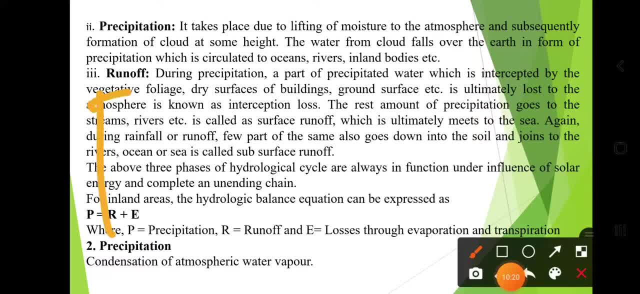 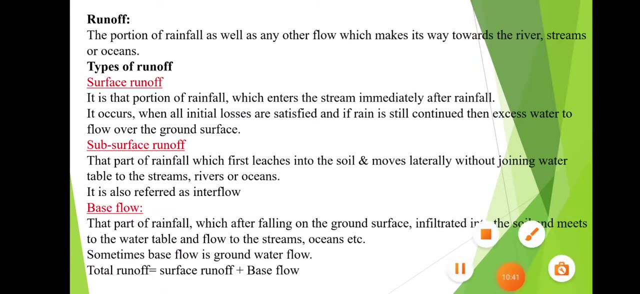 Means. P equal to P means precipitation equal to runoff, plus E means losses through evaporation and transpiration. Evaporation and transpiration, where P is the precipitation, condensation of atmospheric water vapor, then runoff. There are different types of runoff. Define runoff: 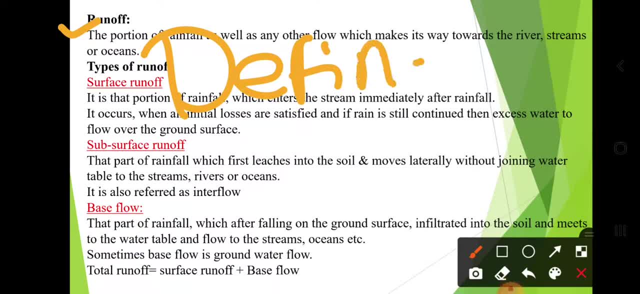 Give the date, What is the definition of the runoff? Define runoff, Then what is runoff? Runoff? it is the portion of rainfall, as well as any other flow, which makes its way towards the streams, rivers and ocean. Then runoff is divided into three types: surface runoff, subsurface runoff and base flow. 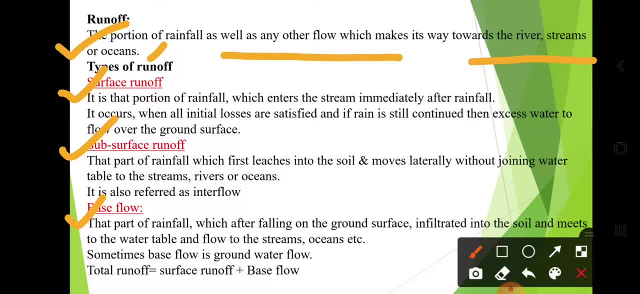 This runoff types are given by the Scientists as per the time delay between the start of the rainfall and end of the rainfall. Okay, When the rain is starting, What happens after the rain starts? Rain starts. Rain starts after a lot of days. 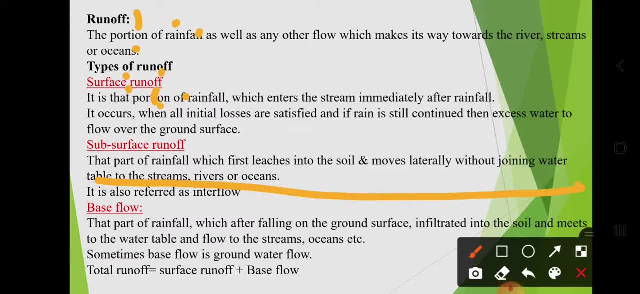 What happens after the rain starts? The land was very dry, The entire surface was dry. When the rain is falling, then what happens? The soil? it will absorb more and more moisture. What happens after a lot of days? What happens after a lot of days? 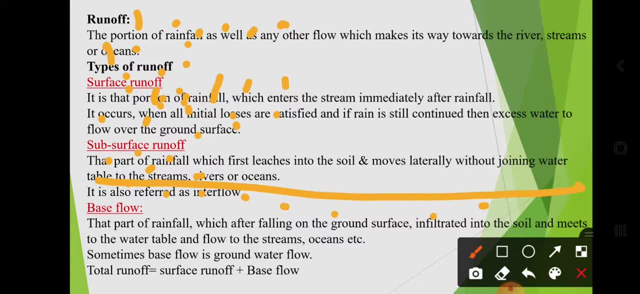 The soil was very dry. The temperature is very high. That is why the rain has absorbed more and more moisture. This is the first entry of water. This one is rainfall after rainfall. What happened? The first entry of water into the soil. it is called as an infiltration. 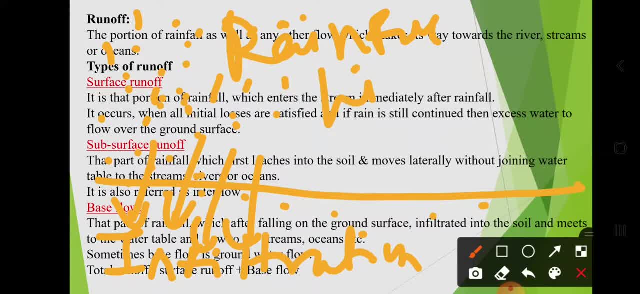 After infiltration, still, rain is falling with high intensity. Rainfall intensity is high. It is raining heavily. The rain스럽 is: they are falling heavily, Rainfall intensities is high. Then, after infiltration, what happened? Each and every pore space is in the soil. it is filled by the water. 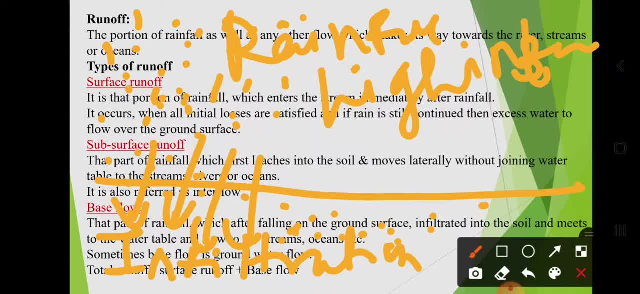 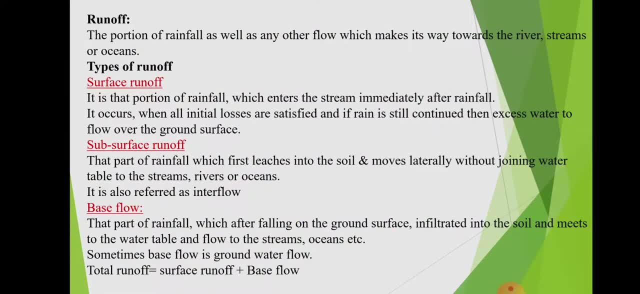 The soil which was in our soothship, the soil which had air in it. it is filled with water. What happens to soil? What happens to soil? Saturated soil? The soil becomes fully saturated, Just like we drank one glass of water, two glasses of water the the soil becomes fluid. 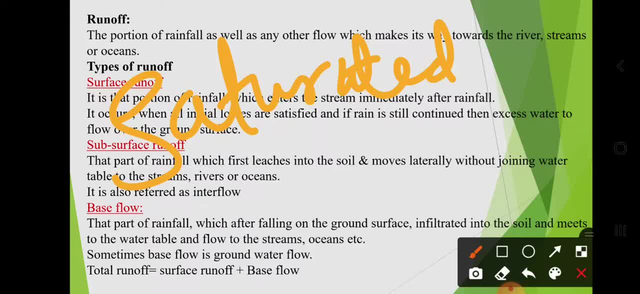 It becomes aerkt, The soil is getting saturated. If we drink 3 glasses of water, then we don't have the capacity to drink the fourth glass. Similarly, the pore spaces in the soil, the air that used to be there, that space has now been taken by the water. 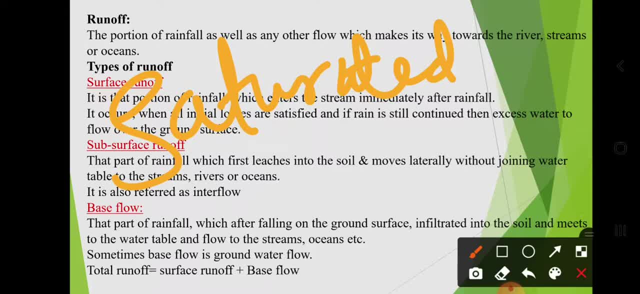 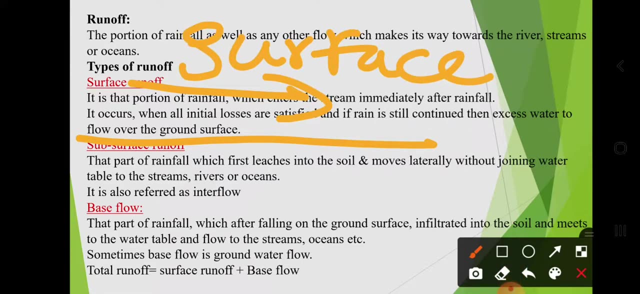 The soil has become saturated with a lot of water. The soil has become completely saturated. now the water cannot enter the soil. This is the way that water is moving over the land surface and it is called as a surface runoff. Now there is very less time delay here. time gap is very less. 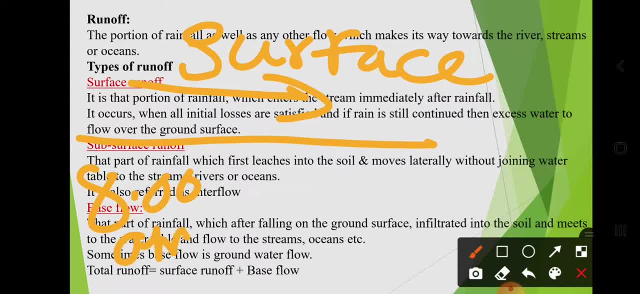 For example, rain is started at 8 am and if the rainfall intensity is higher, if the rainfall intensity is very high, then there will be infiltration and saturation in the soil. It will take very less time because the rainfall intensity is very high and the intensity of rainfall is higher. 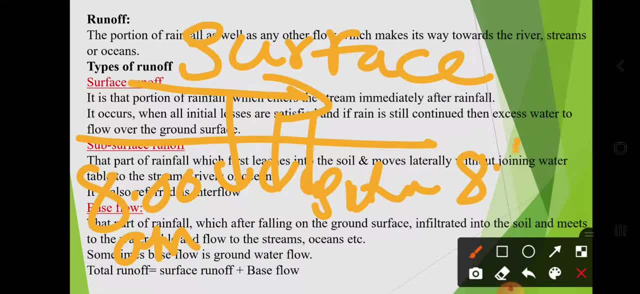 And in that way, 8% of the soil will be saturated. In that way, we will not be able to see the drainage of rainwater in the next 15-20 minutes. It is a 15-minute gap only. maybe depends on the intensity of the rainfall. 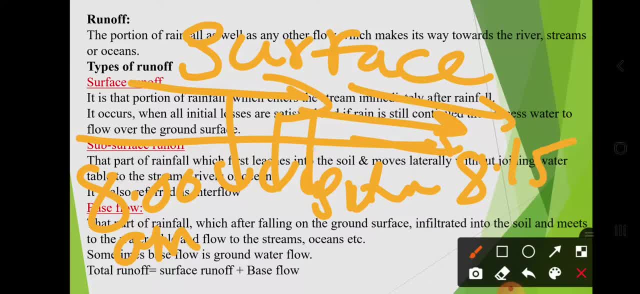 the type of soil, the infiltration capacity, what has been grown on the ground, how the vegetation is attached, all these things affect it, And till then we will not be able to see the drainage of rainwater in front of our eyes. 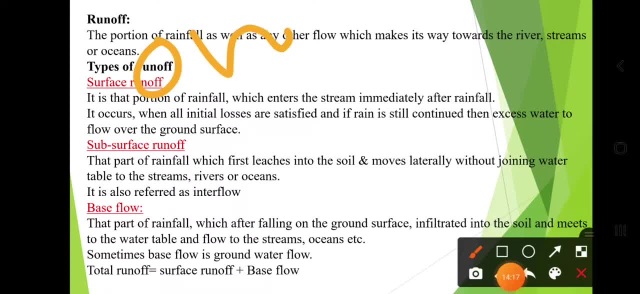 It is called as a surface runoff Or overland flow. Surface runoff is also called as a overland flow. Okay, Means what is surface runoff? Surface runoff means it is the portion of rainfall which enters the stream immediately after the rainfall. 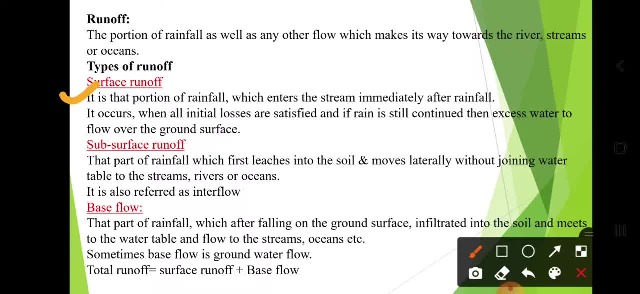 It occurs when all initial losses are satisfied. What are initial losses? Infiltration, Hmm, Infiltration, detention, storage, interception, losses. It is losses. What are solutions? And it is a surface runoff. You see that if the rain is still continuous, the excess water flows on the ground surface. 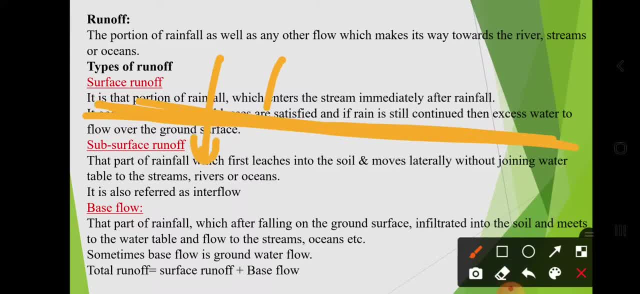 and it is called as a surface runoff or overland flow, Then subsurface runoff. We will be talking about surface runoff. What is subsurface runoff? This one is your ground surface filtration and the soil becomes saturated. We saw earlier that the soil is completely saturated. 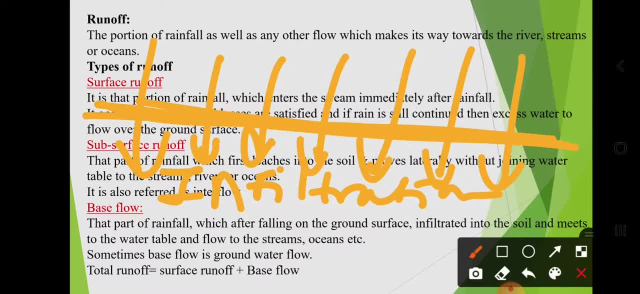 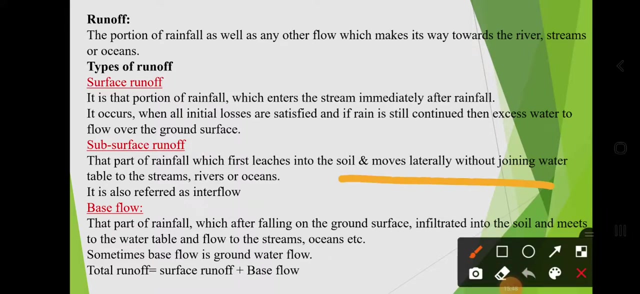 The air is filled with water. Now that water leaches into the soil, It is moving horizontally or laterally below the soil surface. The water- this one- is moving below the soil surface and it is called as a subsurface runoff, Without joining the water table. 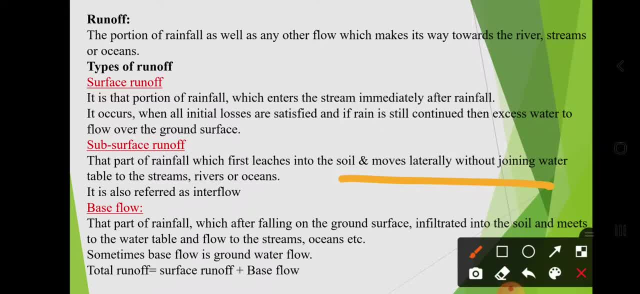 it goes to the rivers, streams and ocean, and it is called as a subsurface runoff or interflow. This infiltrations, however, water which leaches into the soil. This one is your ground surface and whatever the water which leaches into the soil, 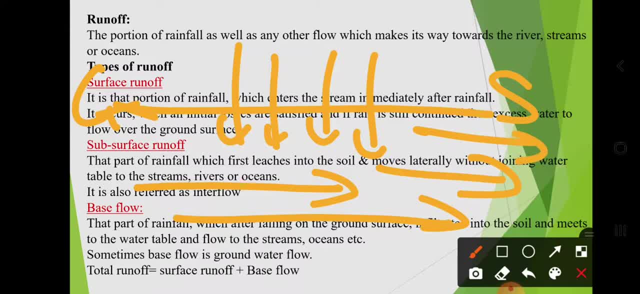 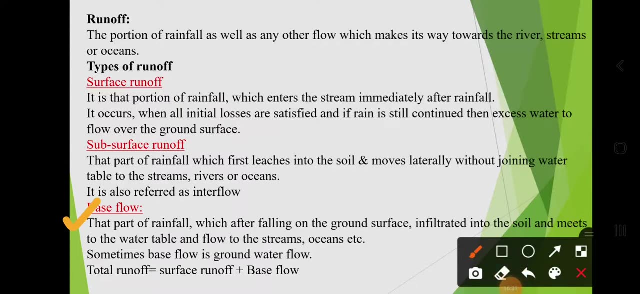 it starts moving Laterally without joining the water table, and it will move towards the streams, rivers and ocean and it is called as a subsurface runoff or interflow, Then base flow, Base flow. Now the time delay is very big here. 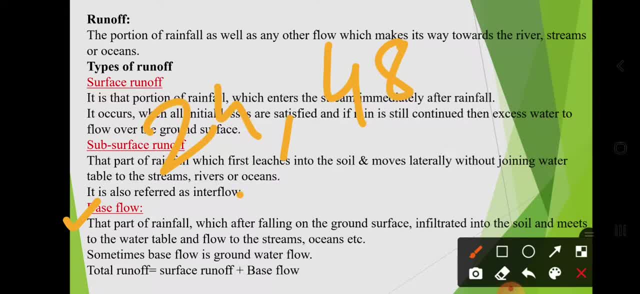 Maybe it will take 24 hours, 48 hours or maybe 72 hours after the rainfall. Pahus padhya nantra chauvi sthasani. it is also called as a delayed flow. It is also called as a delayed flow. 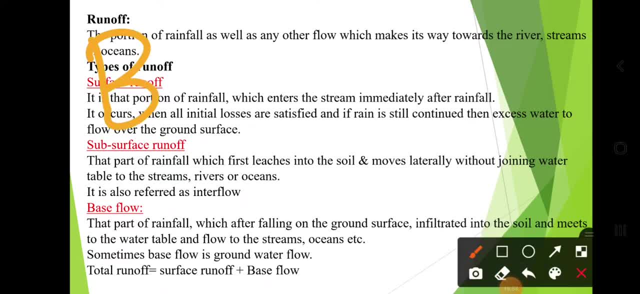 It is very late. Base flow: it is also called as a fill in the blanks which are there. Base flow is also called as a delayed flow Because, whatever the water which is infiltrate into the soil, here the soil is fully saturated. 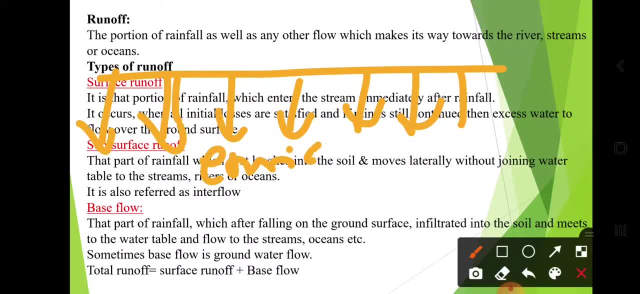 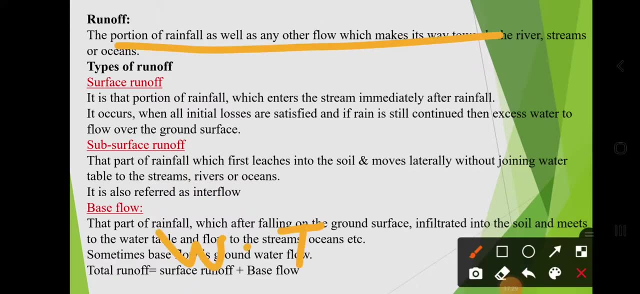 the inner strata. it is enriched by the water and here now the gravitational forces are there And due to the gravitational forces there is a percolation and deep percolation and now water meets the water table. There is a ground water table in Bhugarba. 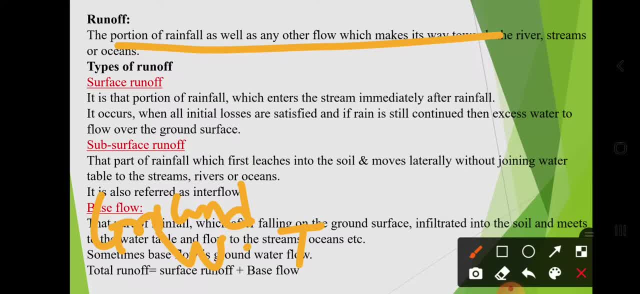 When it is dug up it needs water 50 feet, 100 feet, 150 feet. It doesn't need water on 350 feet Because from the soil we dig up the water. from Bhugarba, the water is drawn directly from the borewell. 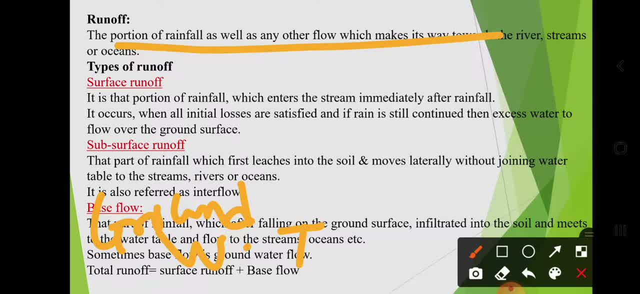 But the water in the soil also needs to be diluted. The soil also needs to be recharged. The borewell also needs to be recharged by harvesting the root water. We don't see this. The water is indeed being extracted from the soil. 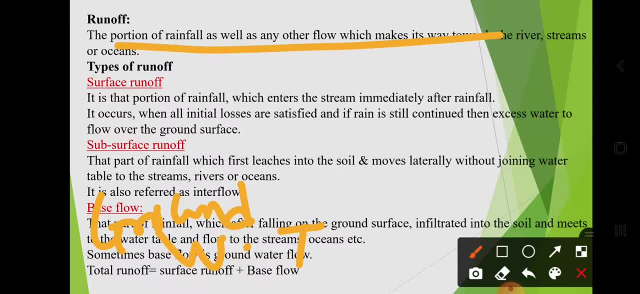 But the water in the soil is not being recharged. That is why the ground water table is reduced by 1 meter every year. Now, in some areas the ground water table is up to 300-300 feet Because, after digging the borewell, 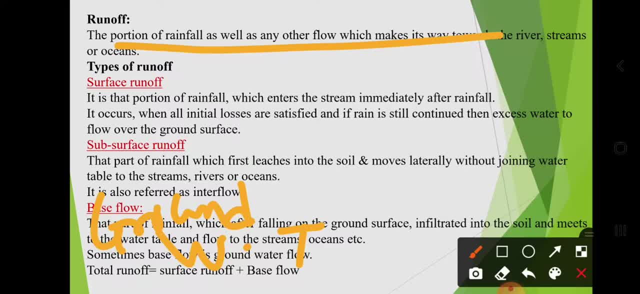 how many feet of water has been used up? We are asking all the questions: 100-200 feet, 500 feet. 500 feet depends on the area. Whatever the ground water table in your area, after digging the well, we will find out. 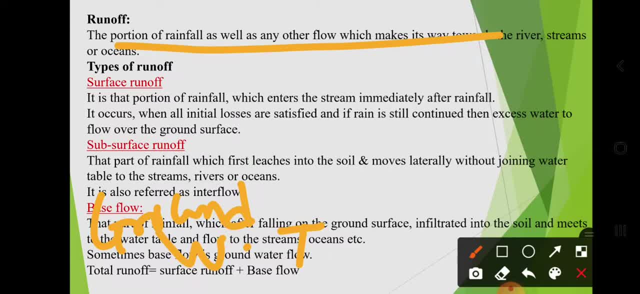 The ground water table is at 100 feet, 150 feet, 300 feet Depends on the recharging. If you are recharging water in your area, there are more soils in your area, more soil and water conservation structure in your area. you will study on that. then the water. 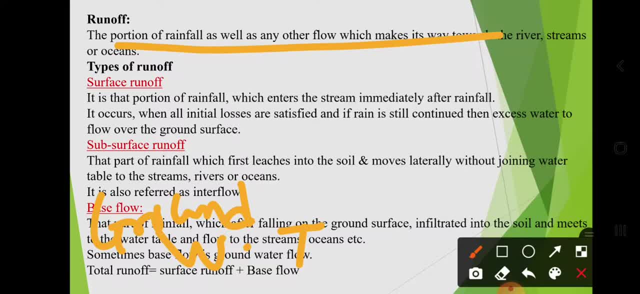 table is at a maybe at less distance, 50 meter, 100 and sorry, 50 feet, 100 feet. but here, what happened now? whatever the water which is infiltrated into the soil, the soil is fully saturated and still the rain is there for a longer time. then what happened? there are the 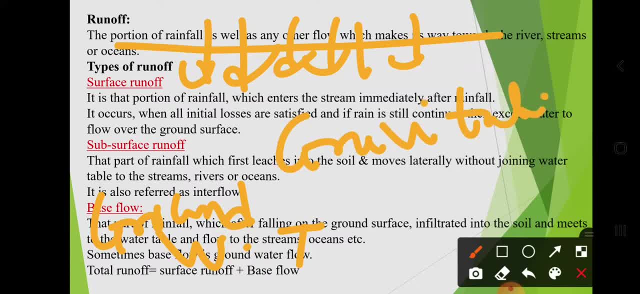 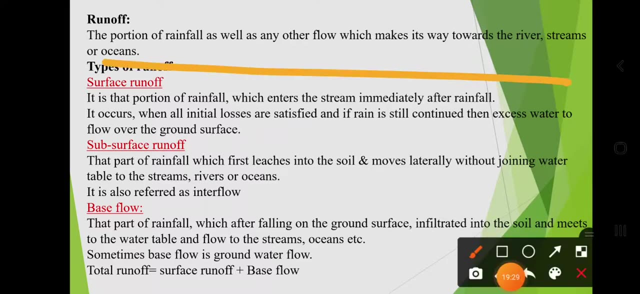 gravitational forces in the ground and due to that gravitational forces, the there is a deep percolation and that water reaches to groundwater table and there is an increase in a level of groundwater table. this groundwater table level goes on increasing because by gravitational forces, there is a percolation, deep percolation, and that water meets to the 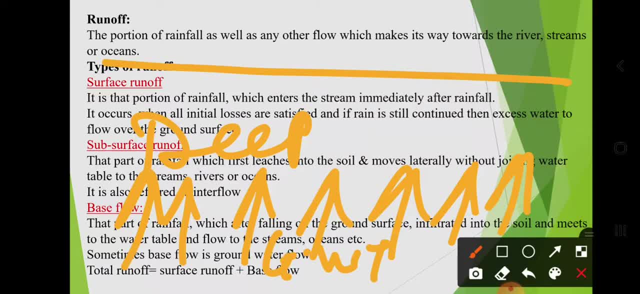 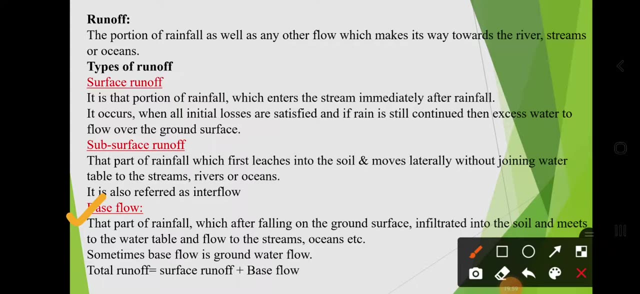 ground water table and increase the level of ground water table. and now that ground water table, it is moving laterally and it is called as a base flow. okay, Base flow means what It is: that part of rainfall which, after falling on the ground surface, infiltrated into the 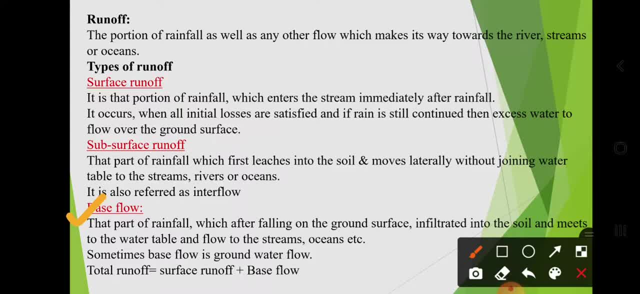 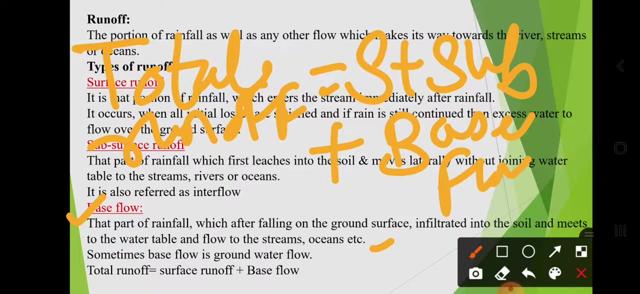 soil and meets to the water table and flow to the streams, rivers and ocean Means total runoff. means what? Total runoff means: surface runoff, subsurface runoff and base flow. The time delay between surface runoff and subsurface runoff is very less. that is why 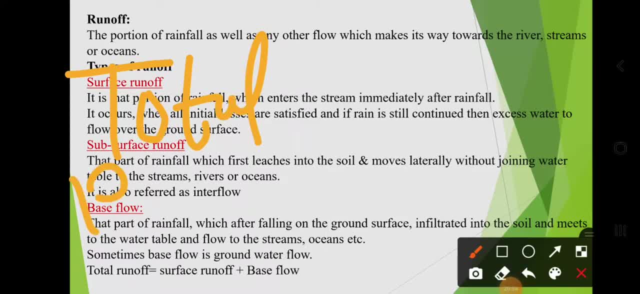 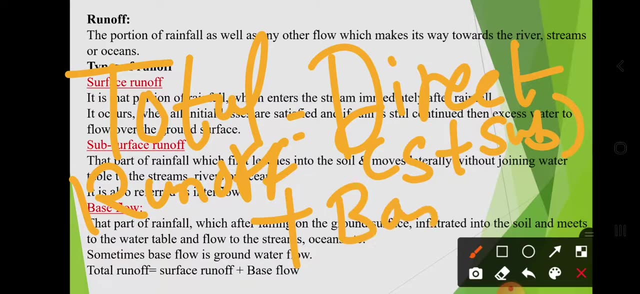 the surface runoff and subsurface runoff. it is called as a direct runoff. Therefore total runoff equal to direct runoff. Direct Direct means surface plus subsurface plus base flow. okay, means total runoff equal to direct runoff plus base flow. total runoff equal to direct runoff plus base flow. 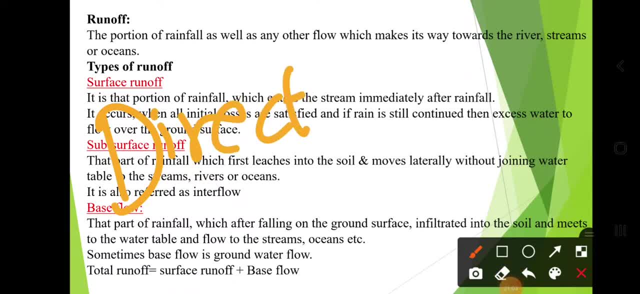 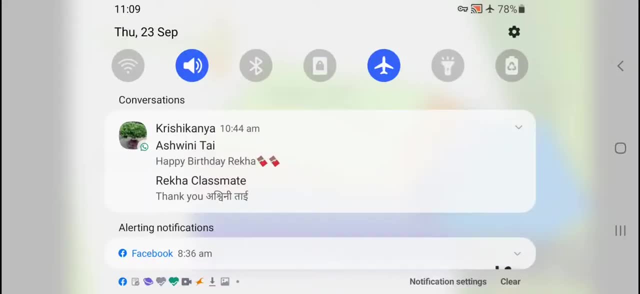 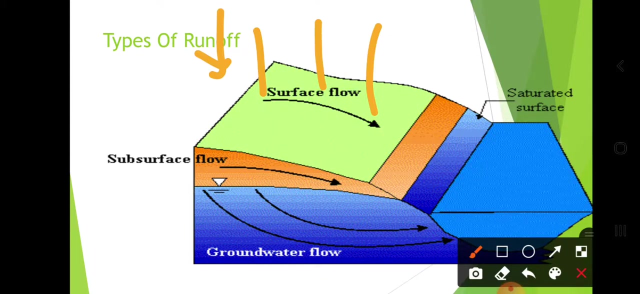 Direct runoff means what? Direct runoff means surface runoff plus subsurface runoff. okay, So this is clear to you. Now see here the diagram. what is surface runoff? After rainfall? there is an infiltration. after rainfall, there is infiltration saturation, and still rain is falling with higher intensity, then water which is moving over the surface. 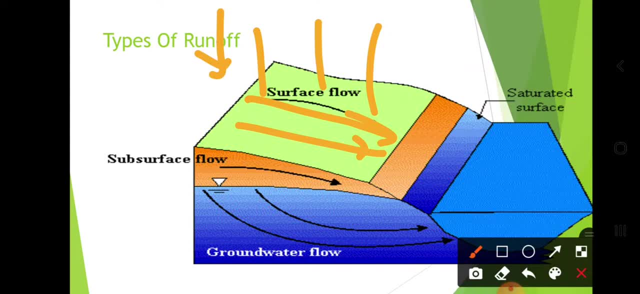 it is called as a subsurface, it is called as a surface runoff, or over land flow, and whatever the water which is infiltrated into the ground, Okay, The infiltrated water leaches into the soil and it will move laterally over the soil surface. 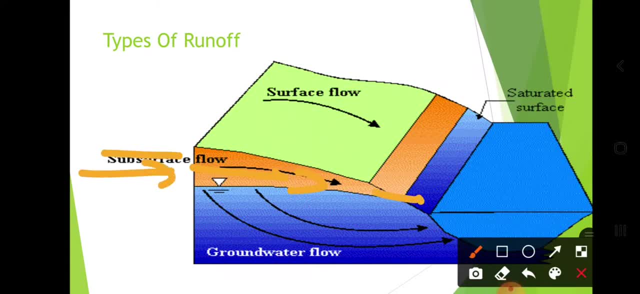 and it is called as a subsurface runoff. It is below the soil surface. that is why subsurface runoff or interflow Now, whatever the water which is infiltrated into the soil, due to the gravitational forces, it will reach to the ground water table and there is increase in a level of ground water. 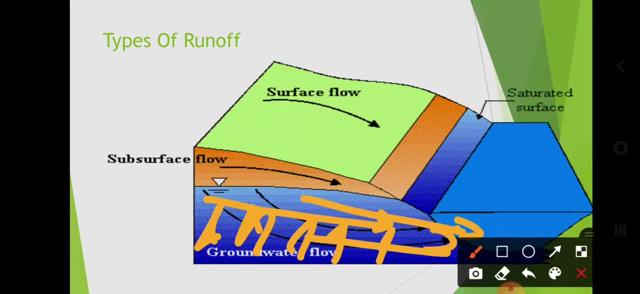 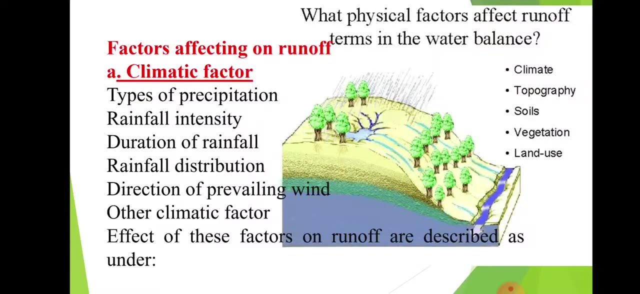 table and that ground water table. it is move laterally and meets to the surface Ocean, sea, ocean, river, sea and ocean and is called as a ground water flow or base flow. Base flow is also called as a delayed flow or ground water flow. 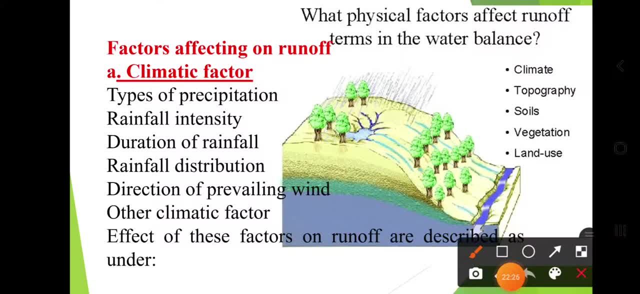 Now, what are the factors affecting runoff? There are 2 types of factor: physiographic factor or climate. In that CSVT, What are the factors affecting runoff? Physical factors affecting runoff: C- Okay, C means climatic factor, S means soil factor, vegetation and topography. 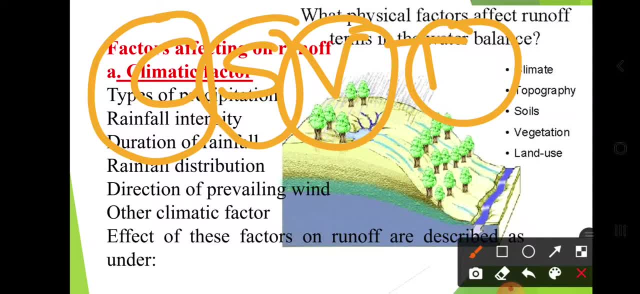 What are the factors affecting runoff? Prajnavicharvajal Parikshamade Explain: define runoff, what are different types of runoff and explain the factors affecting runoff. And what are that factors? C is with you, C means climatic factor, S means soil characteristics. 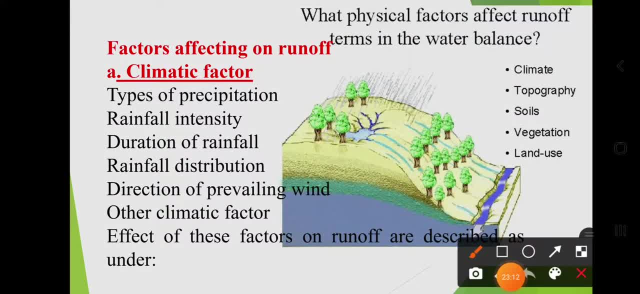 V means vegetation and T means topography, C means climatic factor, S means soil type, V means vegetation and T means topography. Climatic factor in climatic factor. climatic factor is having again type of precipitation. Type of precipitation: if there is a rainfall, then there is more runoff. runoff is more. 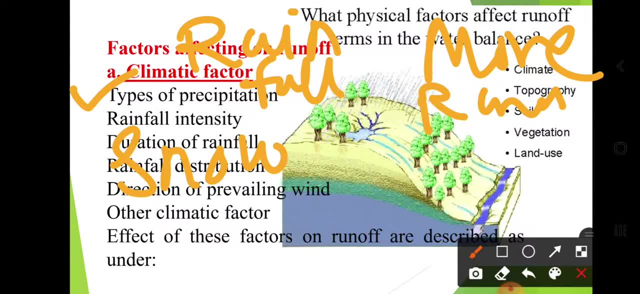 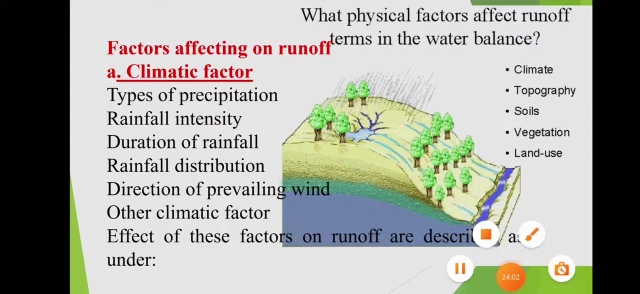 If there is a snowfall, Then snow. there is melting of the snow and within that time there is infiltration. the contact time between the melting and infiltration is there. that is why there is less runoff. Means type of precipitation also affect the runoff. 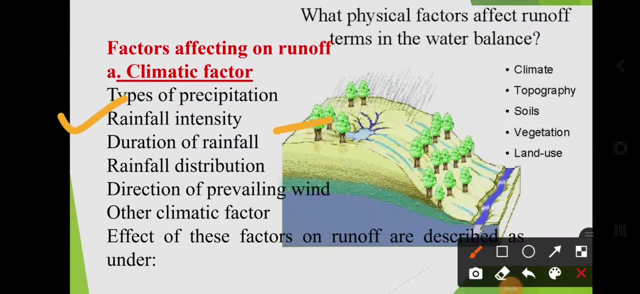 Rainfall intensity. If the intensity of rainfall is higher, then runoff is more. If the intensity rainfall is higher, then runoff is higher. If the intensity of rainfall is higher, then runoff is more. The intensity of rainfall is less, then runoff is less. 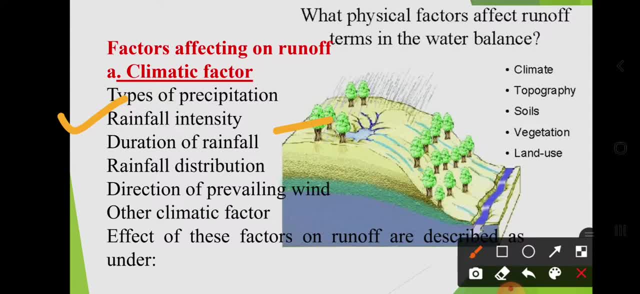 The rain is very heavy. there is a lot of runoff. The rain is very heavy. the intensity of the rain is less. there is a lot of rain, Then what will happen? More and more infiltration will happen. the soil will remain wet. then there will be less runoff. 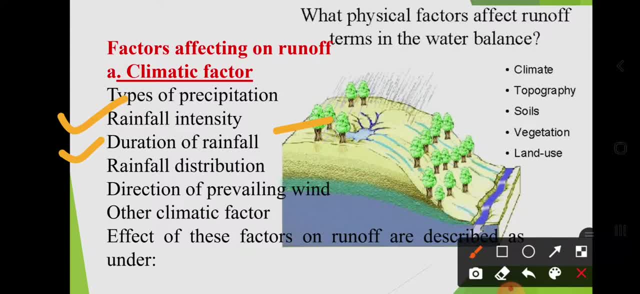 Duration of rainfall. If the rainfall duration is very less, then runoff is less. If the duration of rainfall is more, there is a lot of rain, then there is a lot of rain, There is a lot of runoff. Distribution of rainfall. 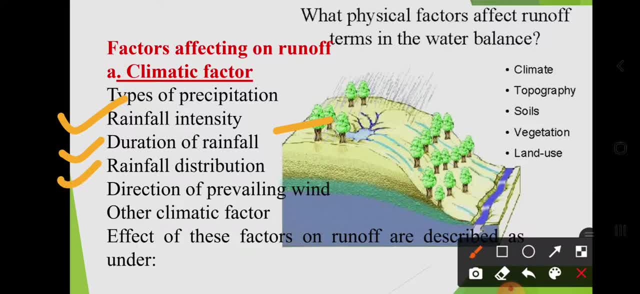 If the rainfall distribution is uneven then it also affects the runoff Direction of prevailing wind. There is a lot of wind and there is a lot of rain. Maybe there is more runoff towards the wind direction. Other climatic factors- effect of these factors on the runoff are described under: 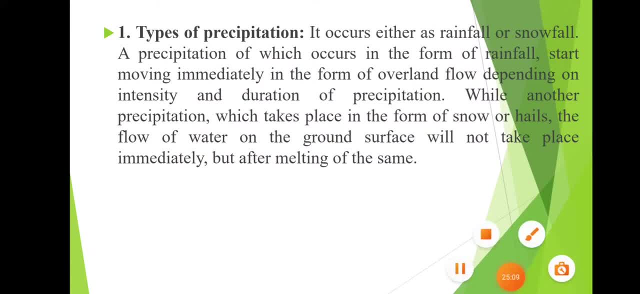 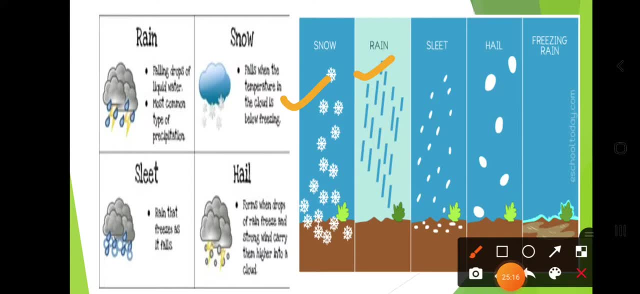 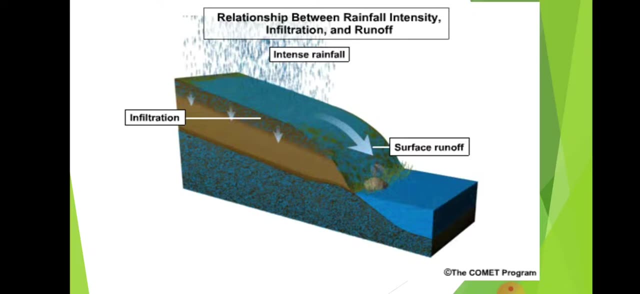 Okay, Then type of precipitation. There are different types of precipitation: Snow rain, sleet, hail and freezing rain. Okay, these are different types of precipitation. It will affect the runoff as well as erosion Relation between rainfall intensity, infiltration and runoff. 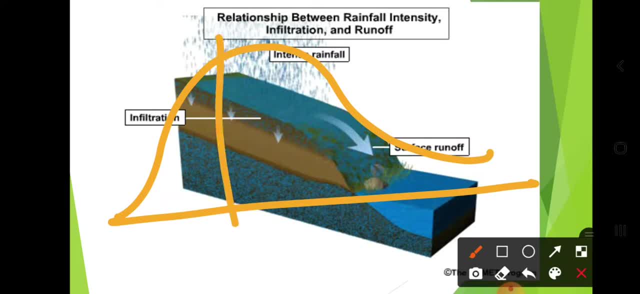 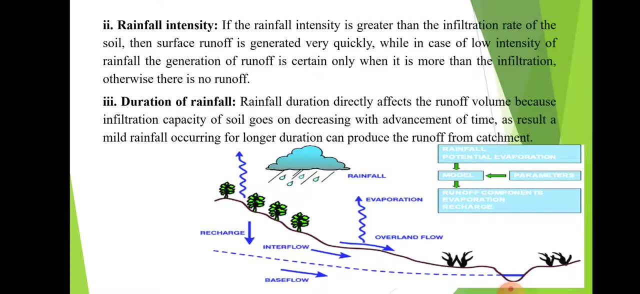 If rainfall intensity is more, then runoff is also more, Then rainfall intensity again. The rainfall intensity is greater than the infiltration rate of the soil, Then surface runoff is generated. The rainfall intensity, The infiltration rate of the soil is less. The capacity of the soil to absorb water is less. 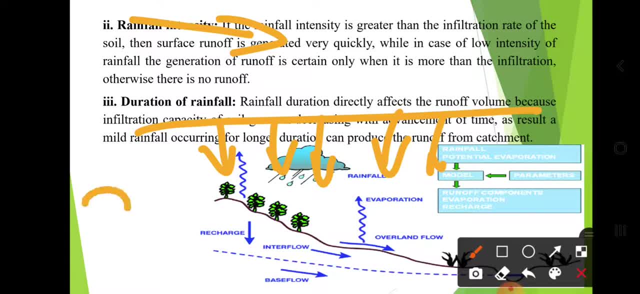 And the rainfall intensity is more. For example, the infiltration rate is 2.5 cm per hour And the sorry mm per hour And rainfall intensity is 5 mm per hour. Infiltration rate is 2.5 mm per hour. 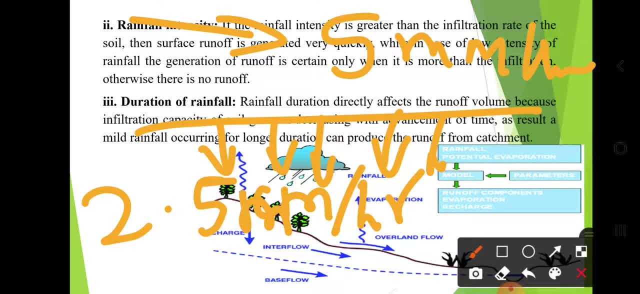 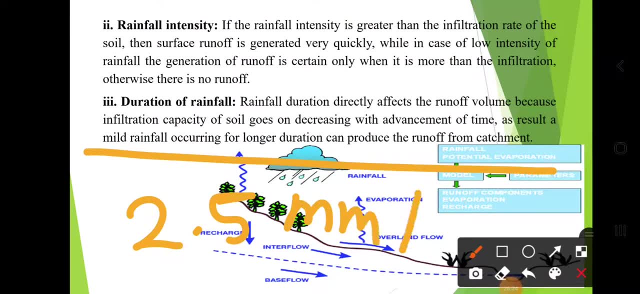 And rainfall intensity is 5 mm per hour Means there is more runoff. But if the infiltration rate is 2.5 mm per hour And rain is 2 mm per hour Rainfall intensity, Then there is less runoff, Means likewise the rainfall intensity. 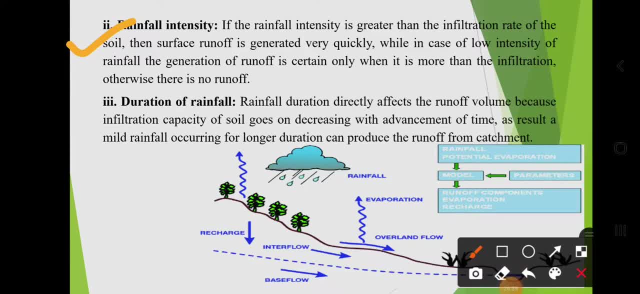 Is greater than Infiltration rate of the soil, Then surface runoff is generated Very quickly, Which, in case of low intensity of rainfall, The generation of runoff is certain Only when it more than infiltration, Otherwise there is no runoff. 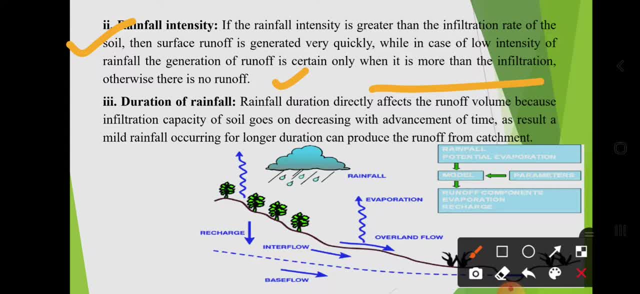 Infiltration rate. In contrast, if there is less rainfall, then there will be runoff Or no, there will be less runoff. Duration of rainfall: How long has the rainfall lasted? Rainfall duration directly affects the runoff Volume Because infiltration capacity of the soil 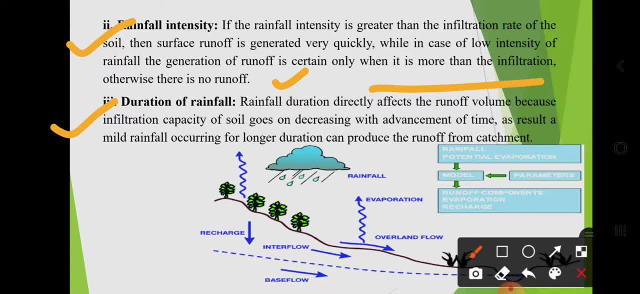 Goes on decreasing with the advancement of the time. As the rain falls, the infiltration rate in the soil decreases And the infiltration rate When the water is completely saturated in the soil, Then there will be no infiltration. The infiltration capacity of the soil decreases. 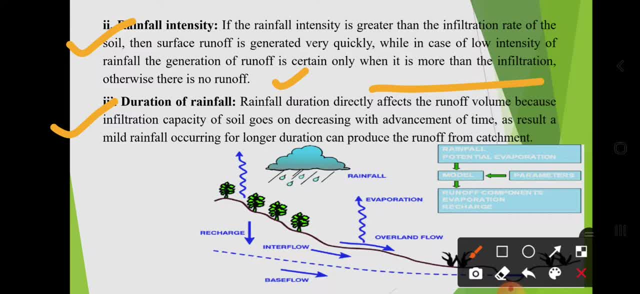 With the advancement of the time, Means as the rain falls. As a result, mild rainfall occurring for longer duration Can produce Runoff From the catchment Infiltration capacity. Purnasali Saturations. However, his or her powers 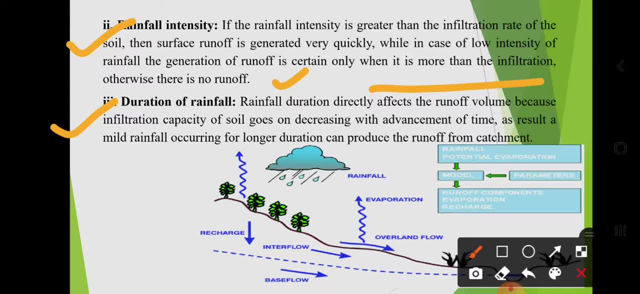 For the same. Thermal runoff on us Means the duration of rainfall. It will affect the runoff volume Because the infiltration capacity of the soil Goes on decreasing with the advancement of time, As a result, mild rainfall occurring for longer time. 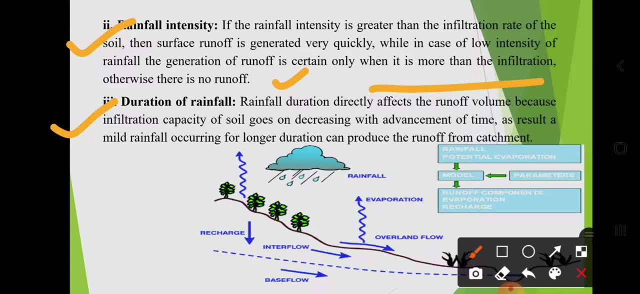 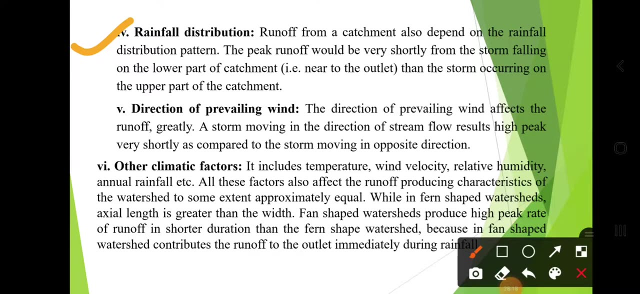 Can produce runoff Still. the rainfall is falling with Less intensity But the duration is more. Then there is a runoff, Then rainfall distribution Distribution from a catchment Also depend on the rainfall distribution pattern. The peak runoff will be very shortly from the storm. 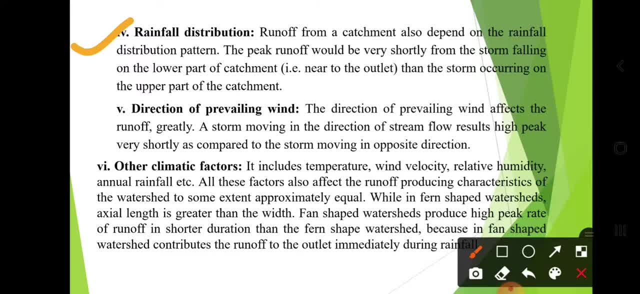 Falling on the lower part of the catchment Than from the storm occurring on the upper part of the crashment Means the distribution of rainfall may be uneven And if the peak It will resume. Peak means highest point Of the watershed. 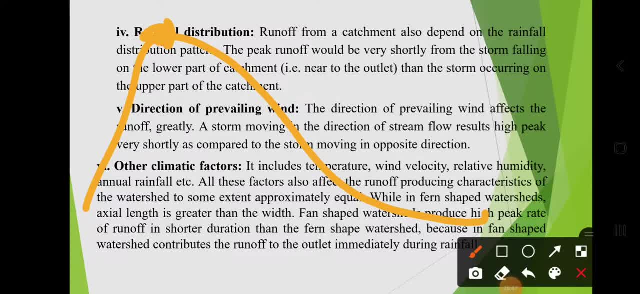 This one is the peak, Highest point of the watershed. It will resume Runoff shortly from the storm falling, Because if there is a rainfall, Then there is a runoff quickly Due to the steep slope Than the lower part of the catchment. 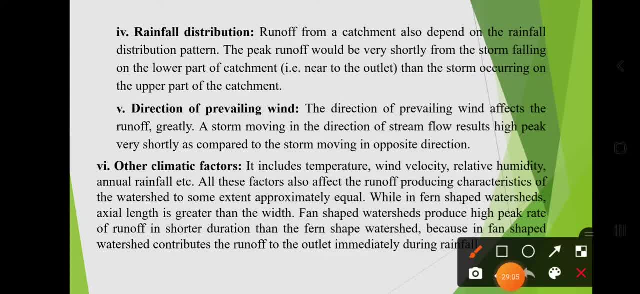 That's why, Then, direction of the prevailing wind. The direction Of prevailing wind Affect the runoff greatly. A storm moving in the direction of stream flow Result in higher peak. The wind is also blowing, The rain is also falling. 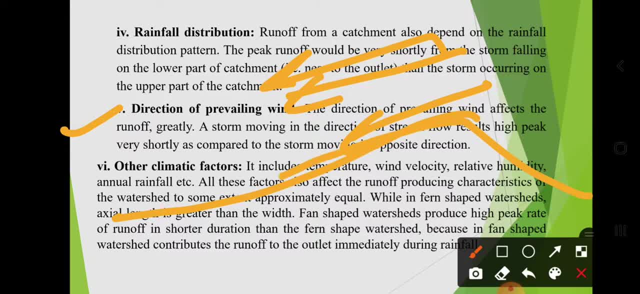 The descent is also in the same direction. Steep slope, The descent is also there. The wind is also in the same direction. The rain is also going in the same direction. Just the wind Likewise Means A storm moving in the direction of stream flow. 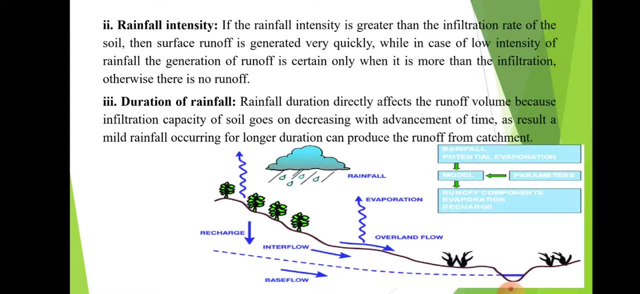 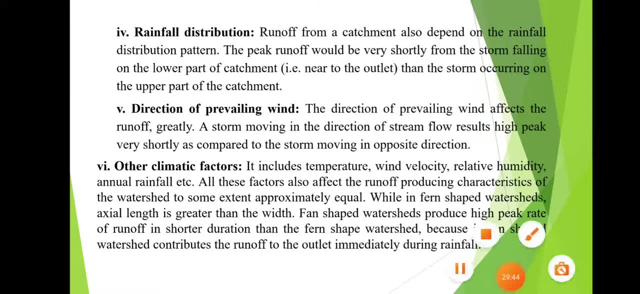 Result: higher peak. Higher peak means This one is a peak Peak. means what Peak means highest point? Peak means highest point, This one is a peak Peak means highest point. Okay, Now other climatic factors. It include temperature. 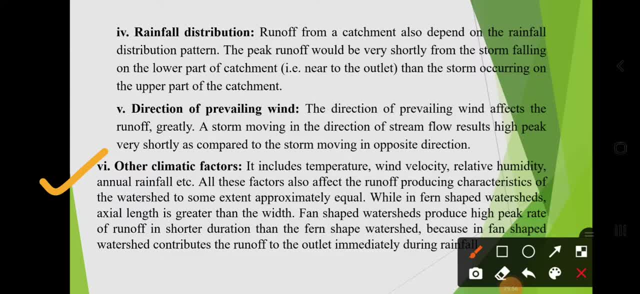 Temperature is high, If it is very hot, If it is raining, Then it will be a little evaporation. Runoff will be less. Wind velocity, Relative humidity, Annual rainfall, All these factors, All these factors also effect the runoff. 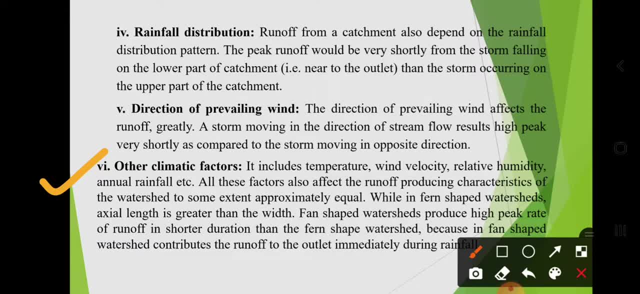 Producing characteristics of the watershed To some extent Approximately equal. While a fern shaped watershed, Now there are different shapes of water shapes: There is a leap shape, There is a triangular shape, There is a circular shape, There is a fern shape, 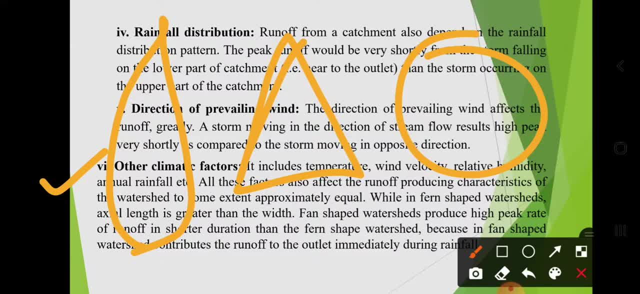 So what is the shape, The area in which the rain is being caught? That is why we call it a watershed catchment area. What is that shape? That is the place at which the rain is being caught, So the amount of rain depends on it. 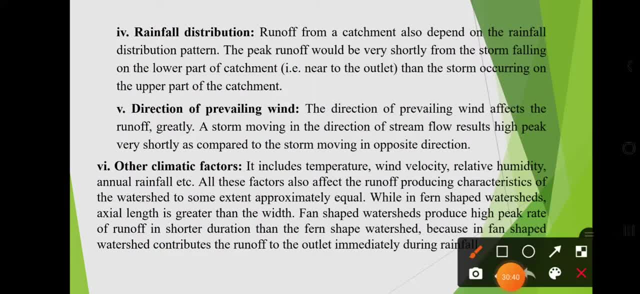 And what does? the scientists says Fern Shape Watersheds: Axial length is greater than the width. Length is more than width. Fern Shape is less than width. Fan Shape Watersheds produce higher peak rate of runoff In short duration. 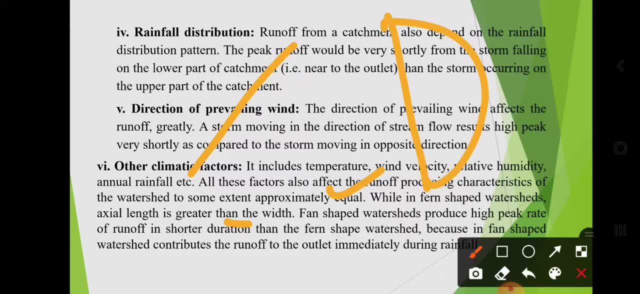 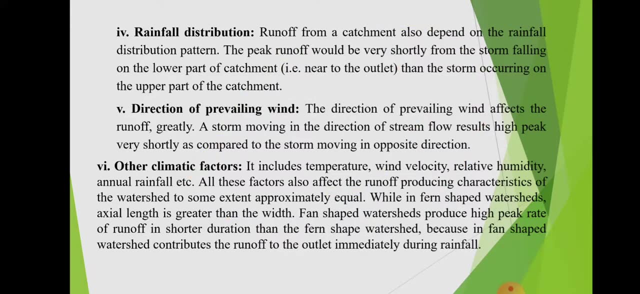 If there are fern shaped watersheds It will produce higher peak rate of runoff in shorter duration Than the paint runoff duration, than the fern-shaped watershed, because in fan-shaped watershed contributes runoff towards the outlet immediately during the rainfall. now this is a physiographic factor, funny watershed. 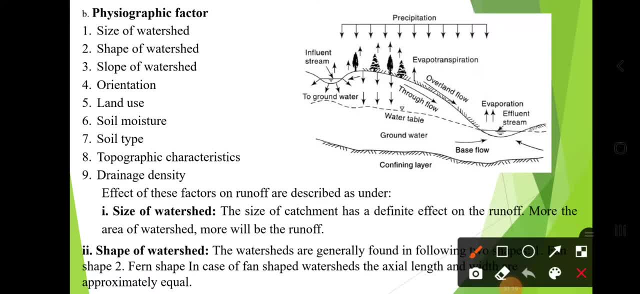 it is called as a watershed. water is catched there. size, soil type, topographic characteristic, drainage density. it will affect the runoff. size of the watershed of the catchment has a definite effect on the runoff. more the area of watershed, more runoff area. just the cell runoff and just the soil. shape of the watershed, shape of the watershed generally. 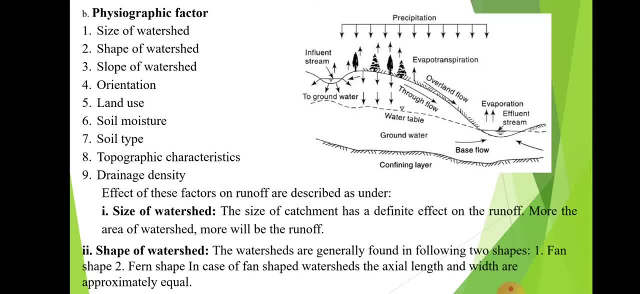 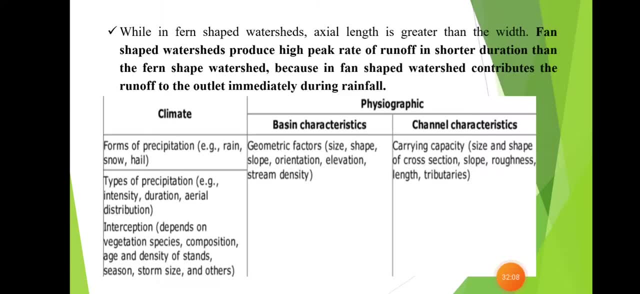 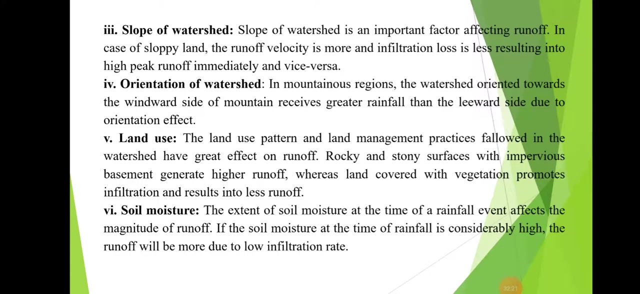 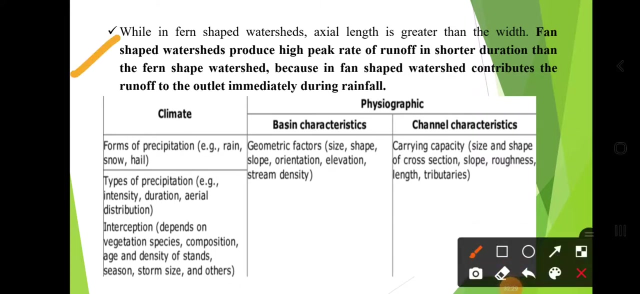 found at two types: fan shape and turn shape. in case fan shape watershed, the axial length and width are approximately equal, while fern shape watershed, having the length is greater than the width. therefore, fan shape watershed produce higher peak rate. fan shape watershed produce higher peak rate in a shorter duration than the fern shape watershed because the farn. 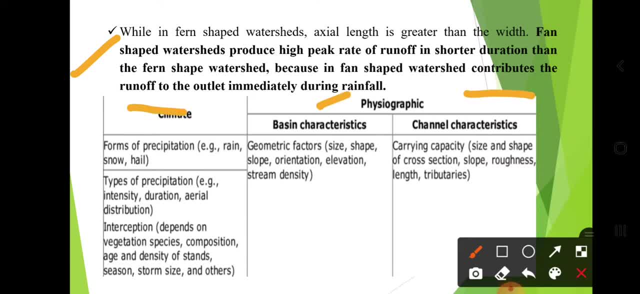 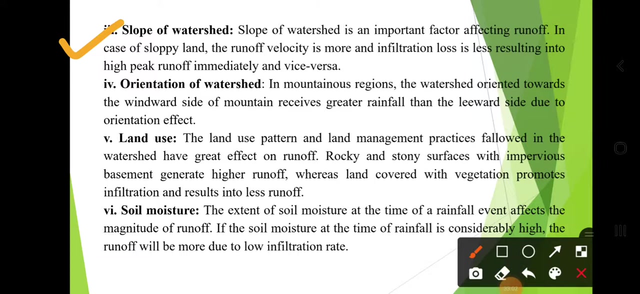 shape. watershed contributes runoff to the outlet immediately during the rainfall they runs. Now there are some climatic factors, basin characteristics and channel characteristics. it will also affect the runoff. The slope of the watershed. slopes are steeper still. Slopey land is still. the runoff velocity is higher. 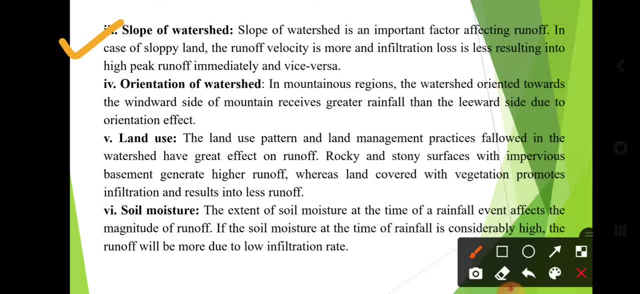 The highest velocity of runoff is there due to the steep slope, and that's why runoff is more. Infiltration loss is less, That's why higher peak of runoff immediately. Then orientation of watershed. In mountainous region, the watershed oriented towards the windward side of mountain receives greater rainfall than the leeward side. 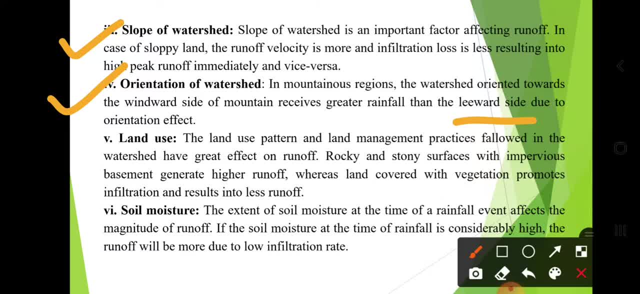 The orientation of watershed is more than the windward side Land use pattern, it will affect the runoff. We will talk about rocky and stony surface. There is higher runoff, Whereas if there is vegetation full of grass, full of trees, the runoff will be less there. 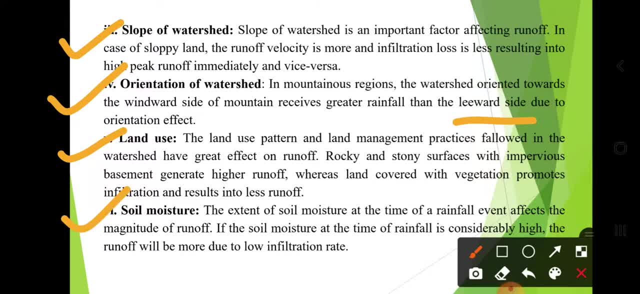 Soil moisture: the extent of soil moisture at the time of rainfall. today it has rained a lot. the soil is completely saturated. Still, if it rains tomorrow, the maximum runoff will be there. That means what moisture was there in your soil before? 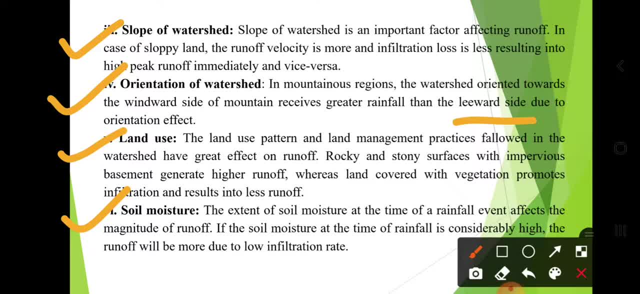 The entire soil is dry, And then, when it rains, there is more infiltration, But the soil is completely saturated. The soil is already wet, The soil is already wet, The water is completely filled And, even if it rains, there will be runoff. 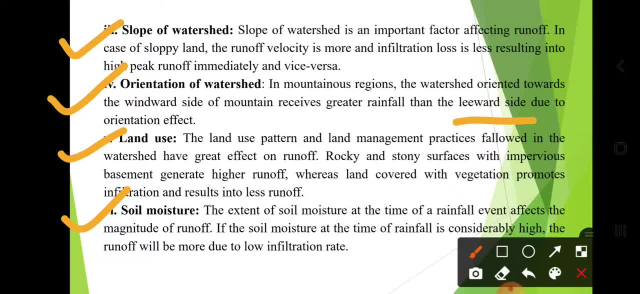 That means the extent of soil moisture at the time of rainfall even affects the magnitude of the runoff. If the soil moisture at the time of rainfall is considerably high, the runoff will be more due to low infiltration rate. Then soil type. Then soil type. 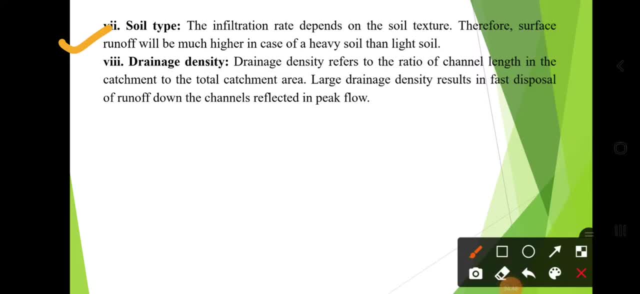 Soil type. the infiltration rate depends on the soil texture. Therefore, surface runoff will be much higher in case of heavy soil than the light soil. Drainage density refers to the ratio of channel length in the catchment to the total catchment area. 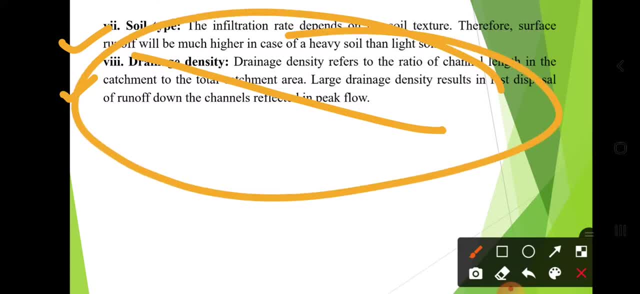 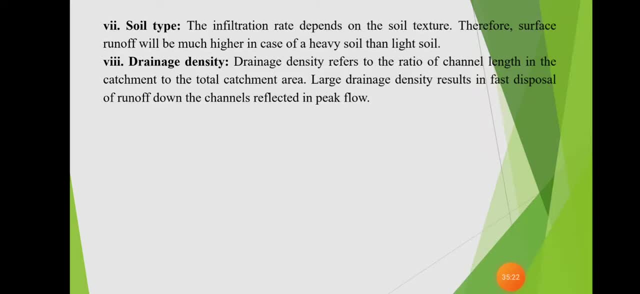 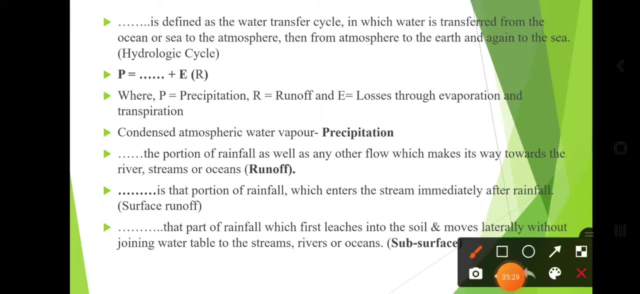 Channel length divided by the total catchment area. Channel length divided by the total catchment area, It is drainage density, It is drainage density. The large drainage density result in fast disposal of runoff down the channel, reflected in the peak flow. Ok, Now there are some objective on that topic.